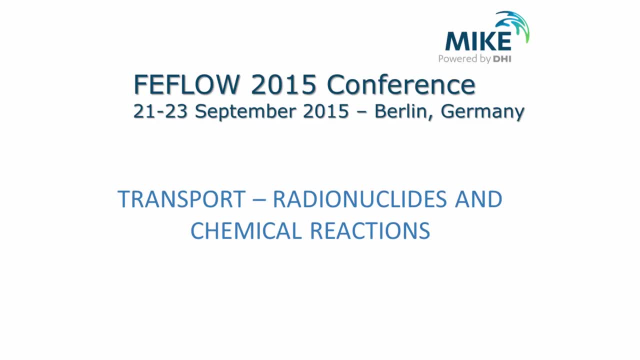 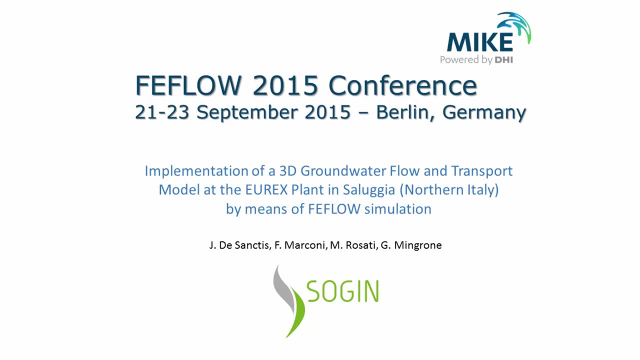 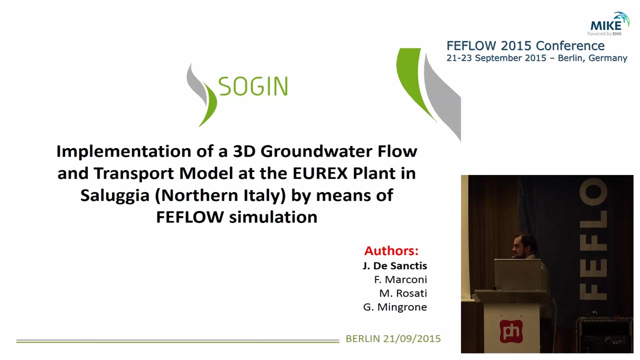 Good afternoon everybody. I am Jacopo the scientist and I'm working with SOGIN SPA, that is a state company in Italy for the commissioning of the whole nuclear power plant and the nuclear waste management. Today I would like to talk about implementation of a 3D groundwater flow. 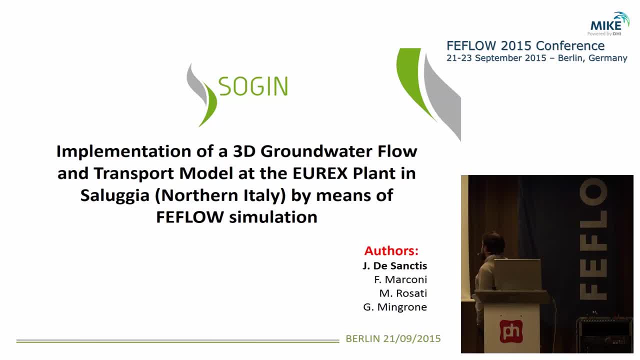 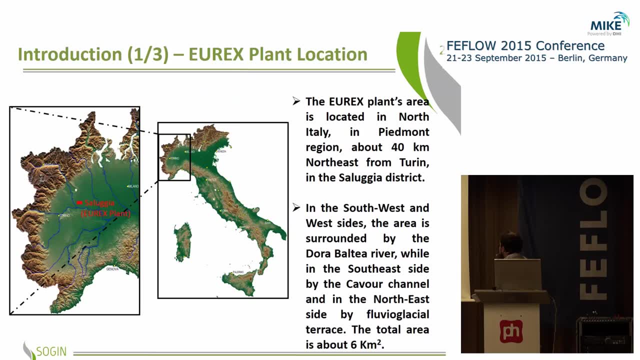 and radionuclides transport model at EREX plant in north of Italy. that means free flow simulation. The EREX plant area is located in Italy in Piemonte region, near Turin. In the southwest and the west side, the area is surrounded by the river. 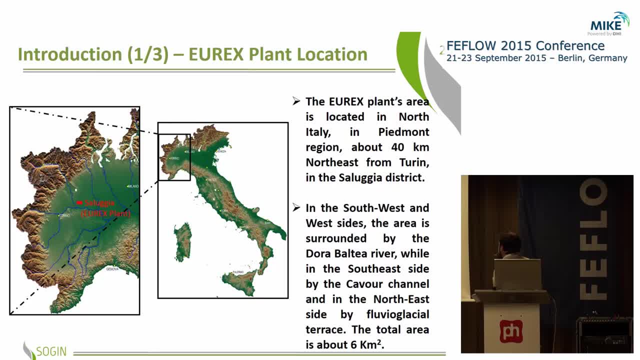 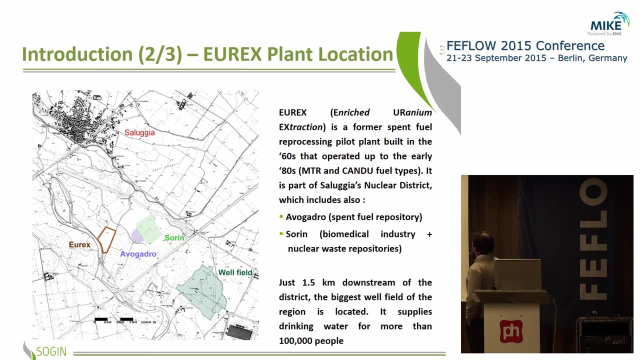 called Dora Baltea, while in the southeast side by the irrigation channel and in the northeast side by fluvial glacial terrains. The total modeling area is about 6 km2.. EREX is a former spent fuel reprocessing pilot plant. 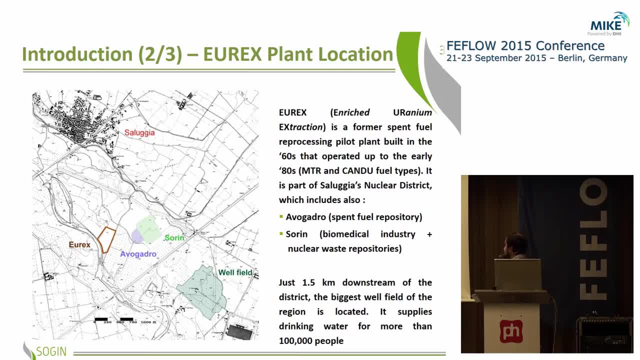 that was built in the 60s. We have another EREX plant. We have two different repositories: Avogadro, that is a spent fuel repository too, and SOGIN, that is a nuclear waste repository for the biomedical industry. 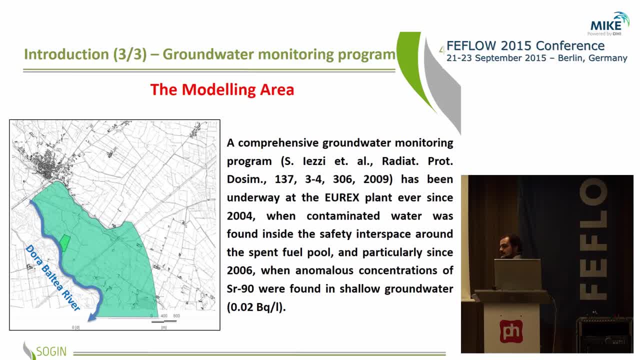 Why we performed the numerical modeling in this area? Because in 2004,, it was found a contaminated water inside the safety interspace around the spent fuel pool And in 2006,, anomalous concentrations of strontium-19 were found in the shallow aquifer. 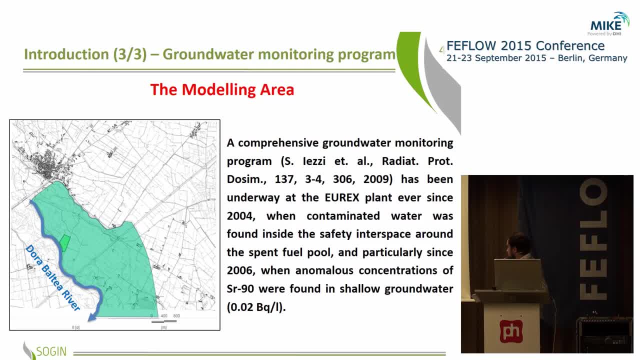 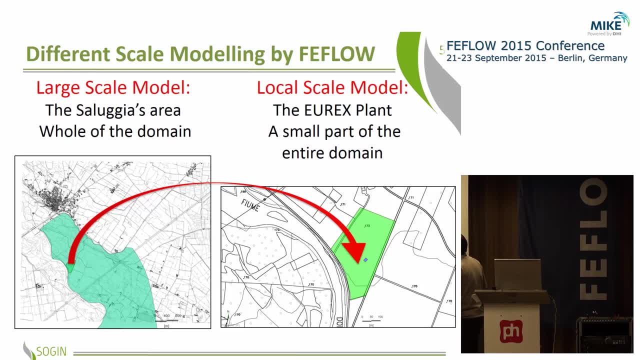 The area, the modeling area is on the left side of this picture And we performed to do this. we performed two different models: A large-scale model that is the whole of the domain, the Saluja areas, and the local-scale model. 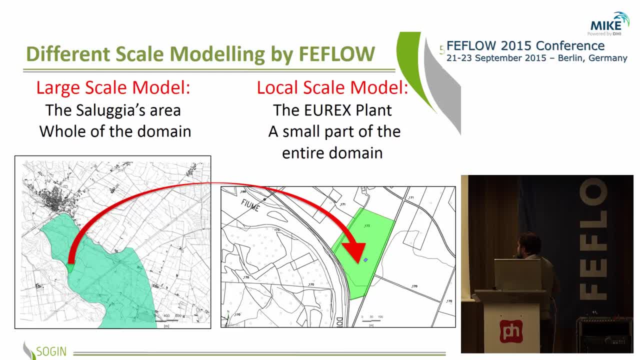 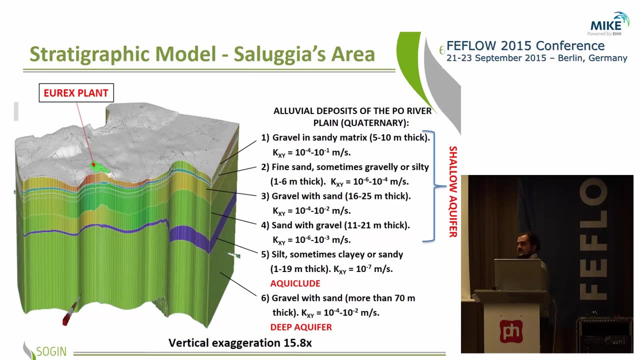 that is a small part of the entire domain. that is only the EREX plane we can see here. The blue area is the pool, the spent pool. By means of many experimental data, hydrological and geological data- we were able to reconstruct: 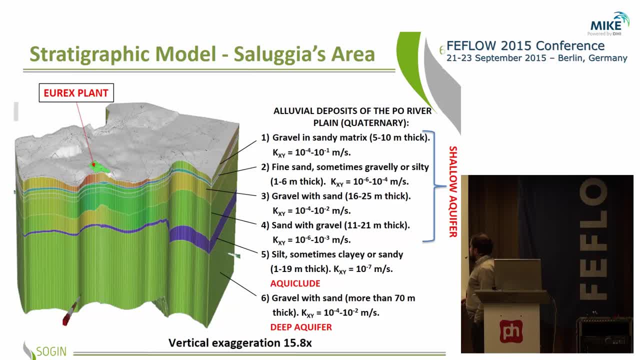 the domain, the stratigraphic model, And we can see six different layers. Each layer is characterized from different porous mediums. The range of porous mediums is here, And the first to fourth layer represents the shallow aquifer. The fifth layer represents the aquaclude. 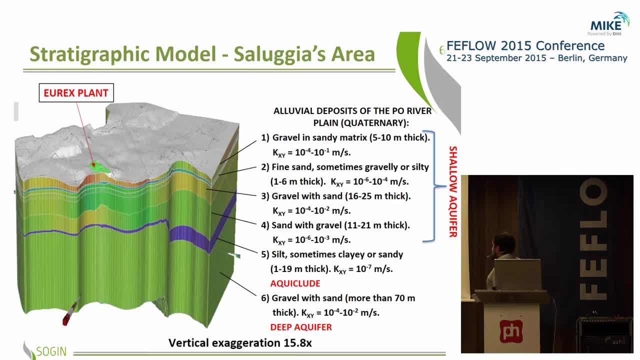 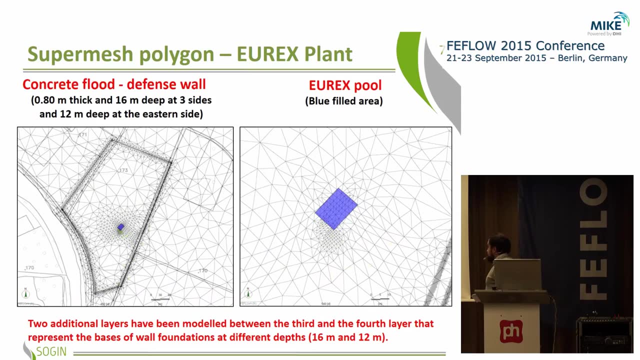 And the last layer is the deep aquifer. Now we modeled only the shallow aquifer as the first application. We had to introduce two different supermesh polygons. The first one is the concrete flood defense wall around the EREX plane area. 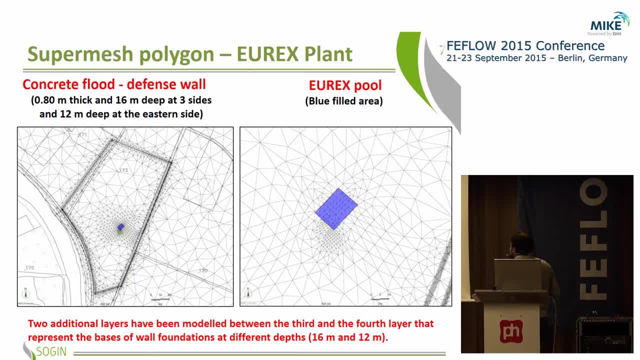 And the second supermesh represents the EREX pool. We had to add two additional layers to represent the basis of the wall foundation, at different depths between the second and the third geological layers. between the second and the third geological layers. between the second and the third geological layers. 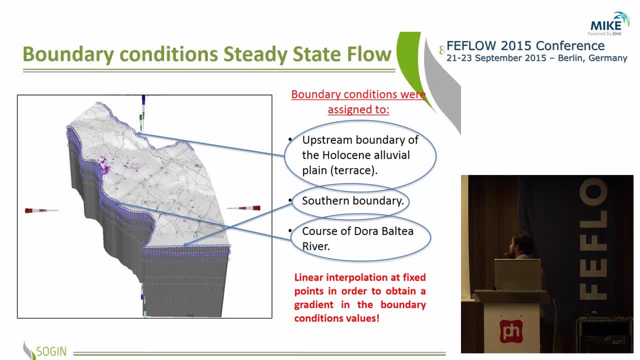 As a first approach, we performed a steady-state flow model. We introduced three different boundary conditions. We introduced three different boundary conditions in upper stream boundary, in southern boundary and for the river. Each boundary condition is a linear interpolation at a fixed point in order to obtain. 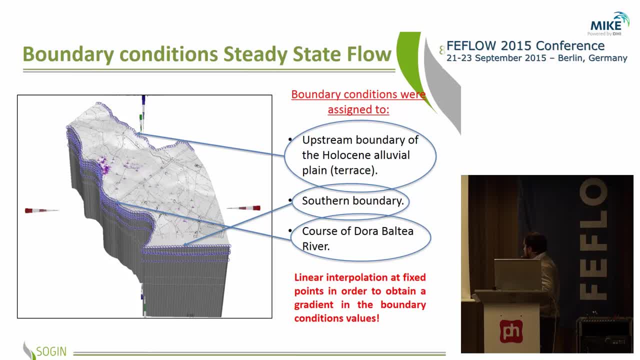 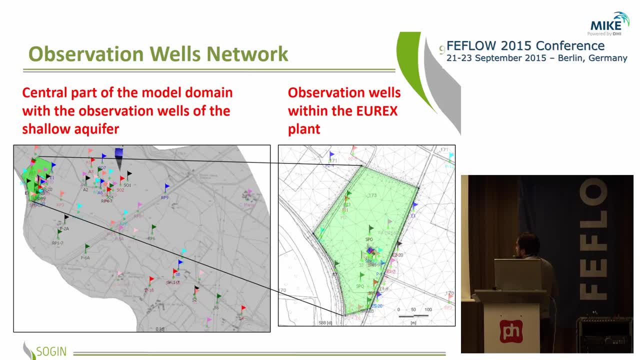 a gradient in the boundary condition value. Here we can see a zoom in a central part of the model domain because we used a great network piezometric observation wells, a great network piezometric observation wells, about 90 wells, about 90 wells, and we can see on the right side. 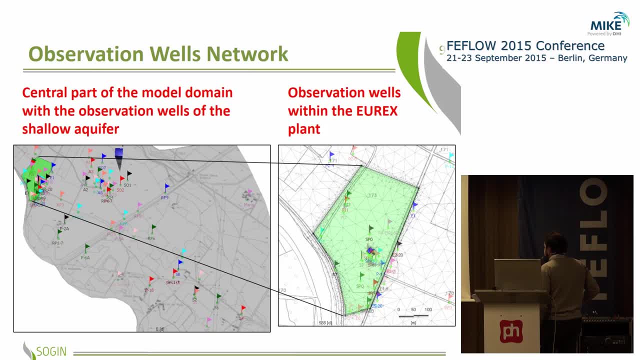 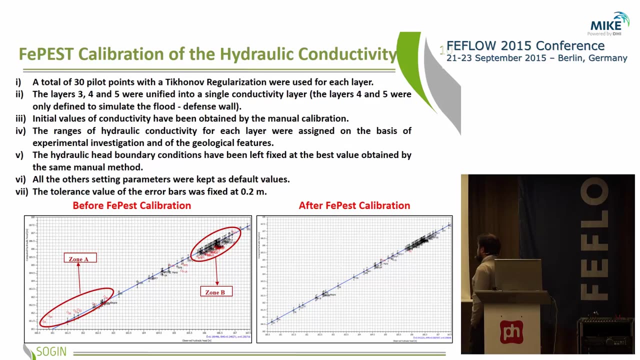 and we can see on the right side the zoom of EREX plane. We have many wells near and close the wall and the pool. Before to use the field-based calibration of the hydraulic conductivity, we performed a manual. a manual calibration only for one boundary condition. 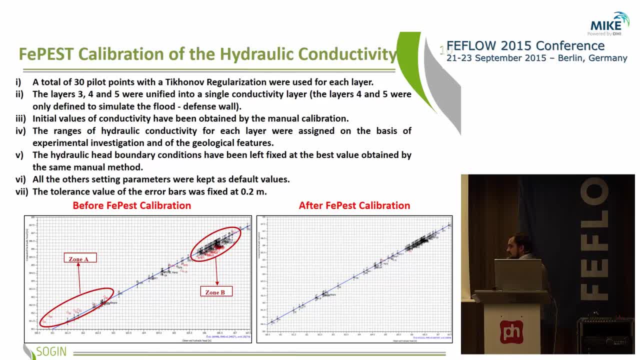 only for one boundary condition, on the north of the domain, Before the field-based calibration, we obtained this situation, this situation that, from a numerical point of view, is a critical situation because we can know two different areas: zone A and zone B. Zone A represents the wells. 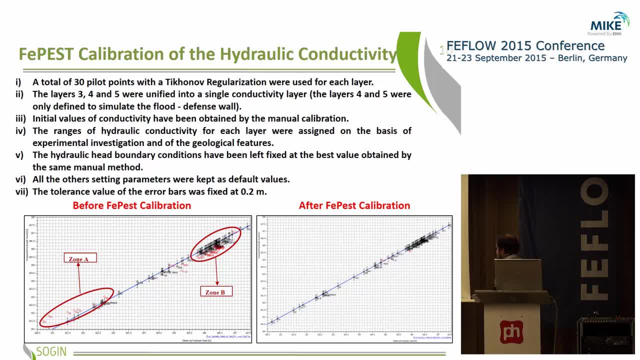 that are located in the south of the domain and zone B, inside the fence wall and around the pool. So a field-based calibration was mandatory. In fact, after the field-based calibration, the scatter plot, that is, the calculated results and the observed data, are in good agreement. 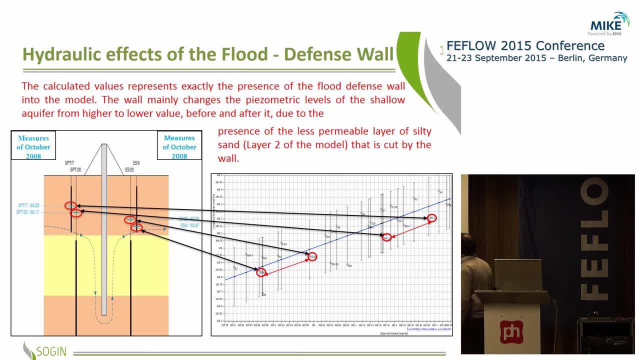 Then our results: the hydraulic effect of the flow defense wall. the main effect of the fence wall is to change the piezometric level of the different wells and the presence of the wall, and we can see the effect here in the calculation. it's important to stress: 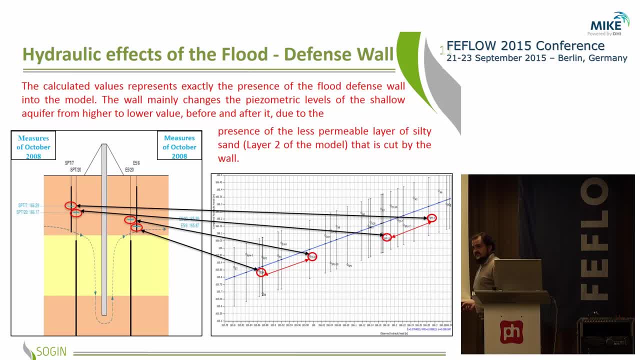 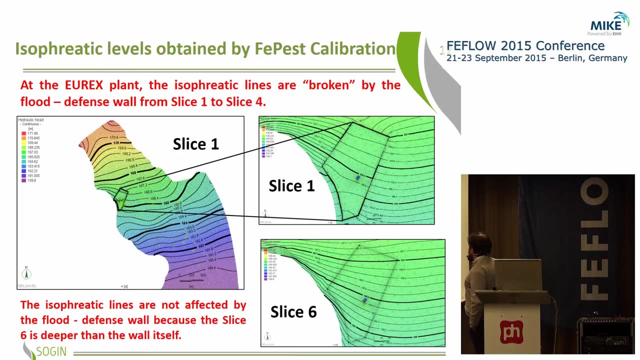 that this effect is independent from the field-based calibration. so the model takes into account very well the hydraulic effect of the wall. Another result obtained after the field-based calibration we can see on the left side of the picture on the slide 1 of the model. 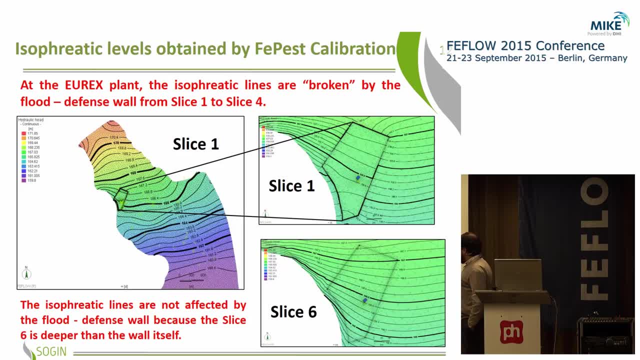 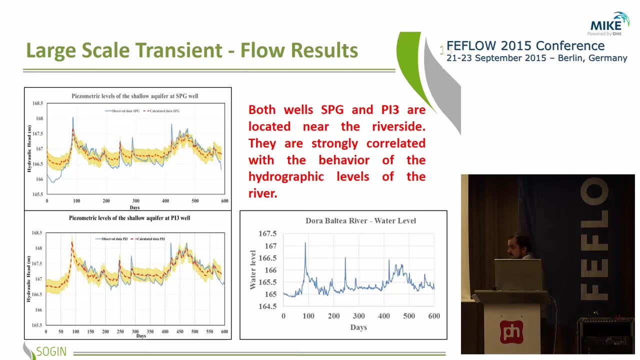 the isofreatic lines that are broken by the wall here, while on slide 6, where the wall, there isn't more than one line. After the steady-state flow, we perform a transit flow simulation. the time of the simulation is about two years. we can see: 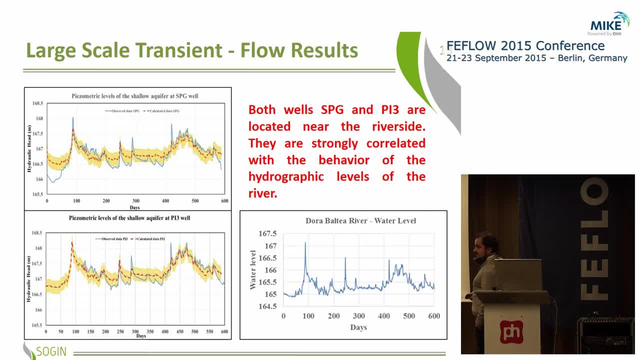 the piezometric level of the shallow aquifer at two different wells, SPG and P3, and the red dash line is calculated by feed flow and the continuous line is the observed data, and we can see that two curves are in good agreement among them. 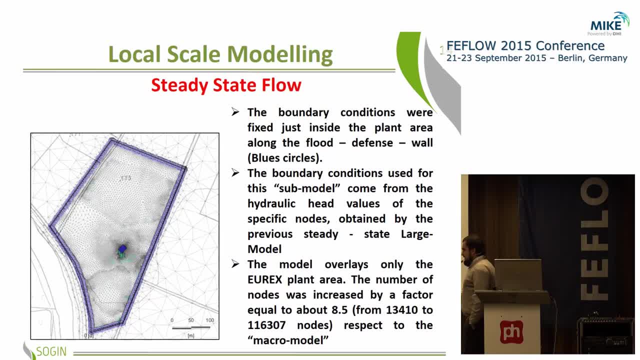 Then to, in order to have lowest uncertainties in the propagation of strontium-90, we performed, I said before, the local scale model and we we had increased the number of nodes by a factor 8.5, from about 2000 nodes to 100 nodes. 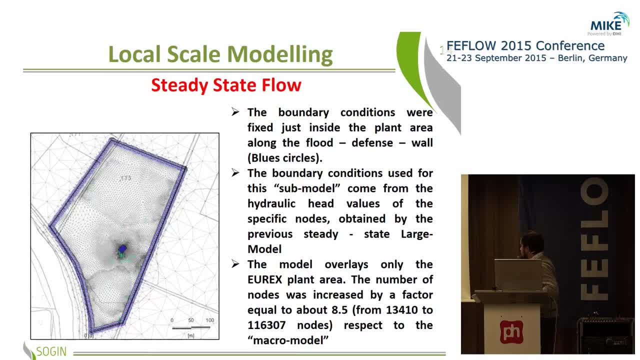 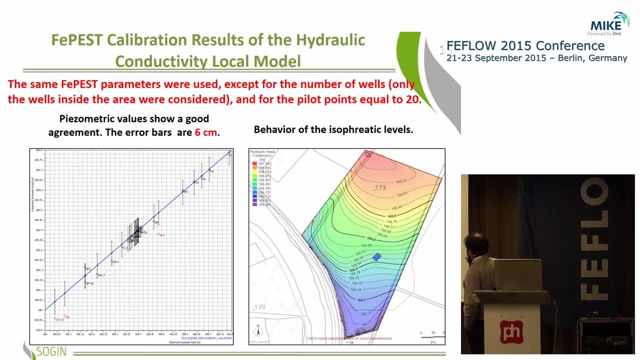 respect to the macro model. we use the same boundary condition calculating the macro model at this point along of the wall, and then we can see here the scatter plot is very, very accurate. we can note the exact agreement between the calculator and the and the observed data in the piezometric level. 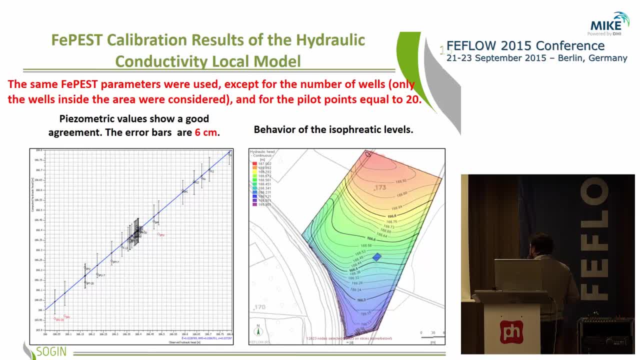 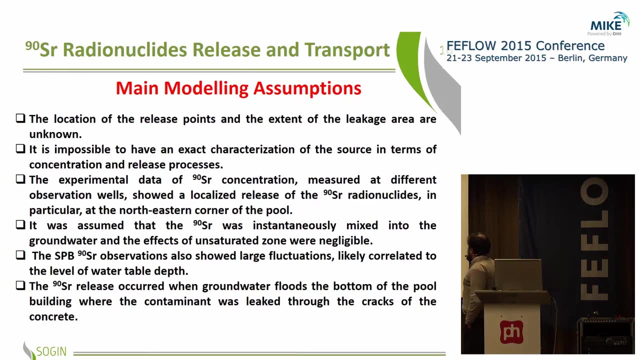 and on the right side we can see a more complex isopriatic line inside the aerox pool. near the pool the error bars are 6 cm of tolerance. then we applied the transport model. we consider only the strontium-90 the main model assumption. 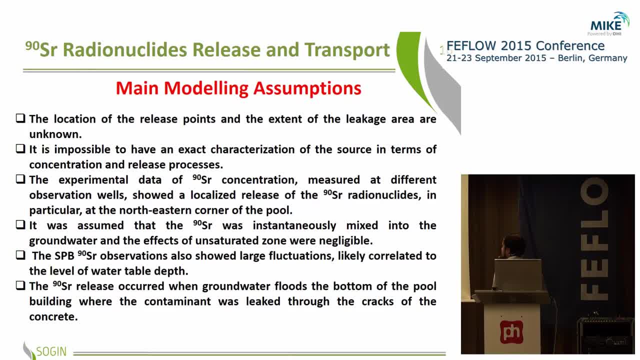 are the following. the most important is that we assume that the strontium-90 was instantaneously mixed into the groundwater and the effect of unsaturated zone. the strontium-90 really is occured when groundwater flows the bottom of the pool building where the contaminant was. 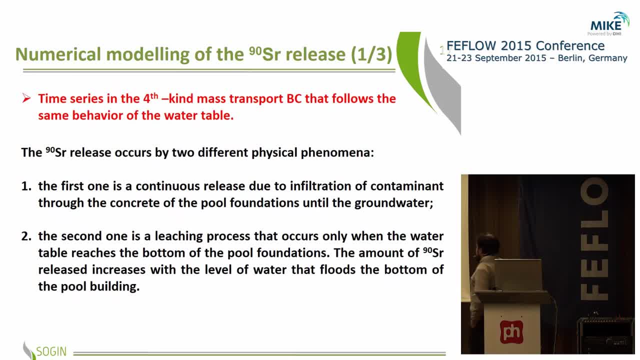 linked to the cracks of the concrete. we used the time series in 40 km mass transport boundary condition that followed the same behavior. the water table. two different main process are considered. the first one is a continuous release due to infiltration of contaminant through the concrete of the pool foundation. 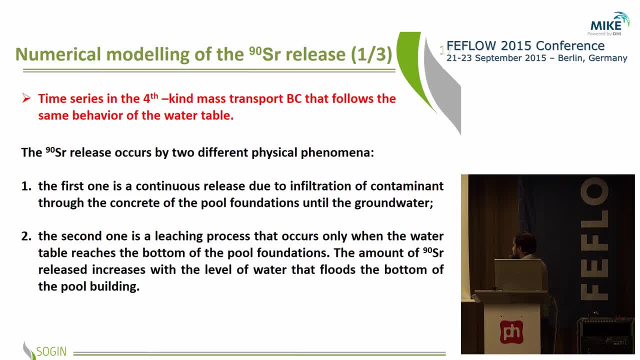 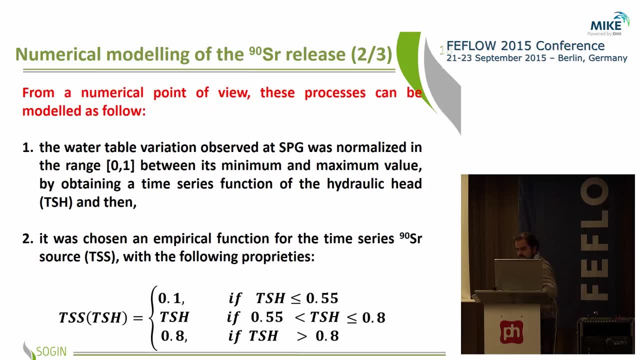 until the groundwater, and the second one is a leasing process that occured only when the water table reaches the bottom of the pool foundation. the amount of 90 strontium released increase with the level of the water that flows the bottom of the pool building we performed 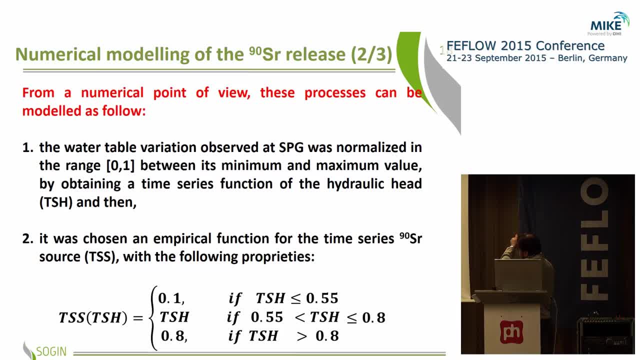 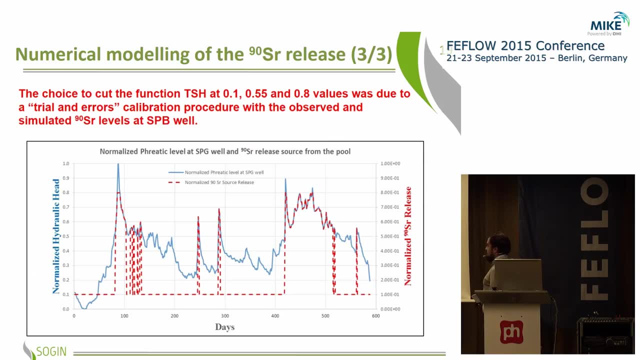 we introduced a function, TSS, that depends of TSH, that is, the level of the water table, is an empirical function that we can see in this picture. the red dashed line is the release of strontium. the horizontal line is the continuous release, while the peaks. 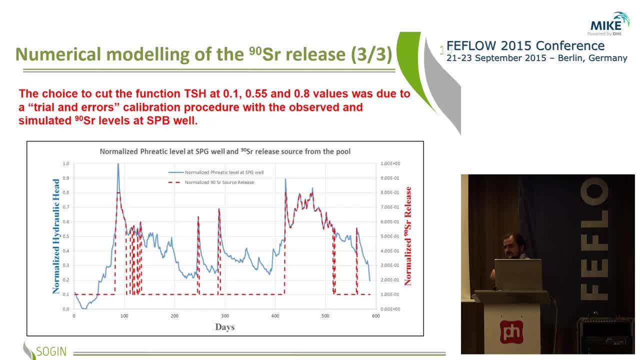 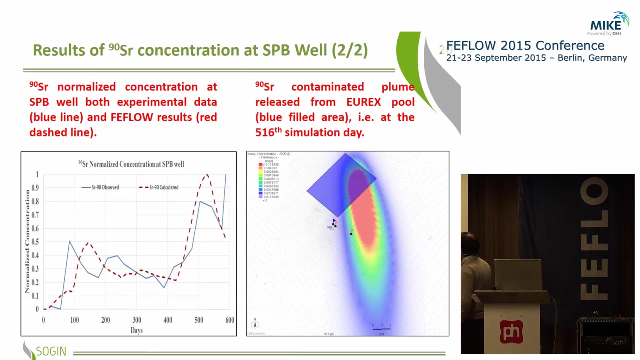 represents the floating of the water, the leasing process of the water in the foundation building and the continuous line is the behavior of the water table. both the curves are normalized with its with their minimum and maximum value for each curve, and is a qualitative study. our results we can see on the right side. 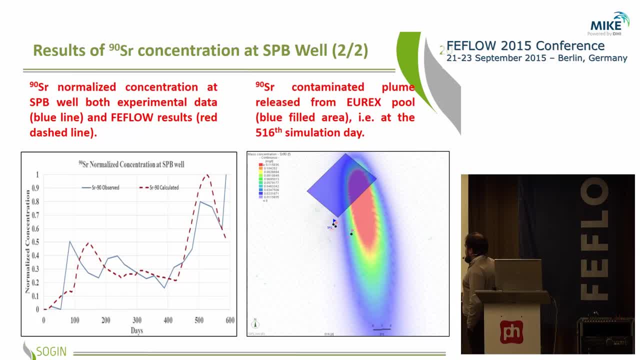 the observed and the calculated curve of the strontium 90 normalized concentration at SPB. well, that we can see here the two curves for our goal as first approach is in a good agreement. and here we can see the two dimensional plot of strontium 90. 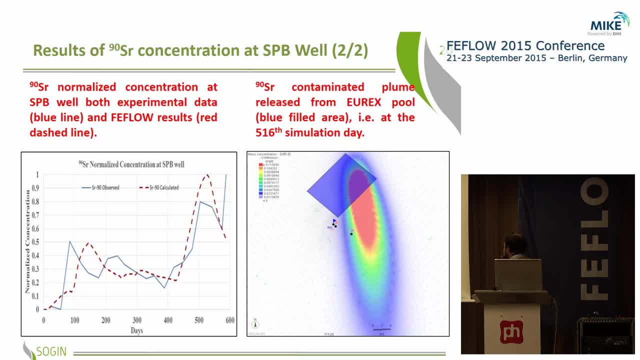 at one simulation day. it's important to stress that here we have two different wells, SPG and SPH, that didn't take any detection of the strontium in the real case, in observation data and in our model, it's the same situation. we can see the same situation. 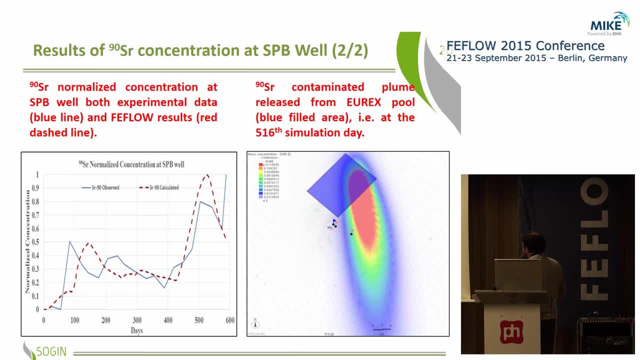 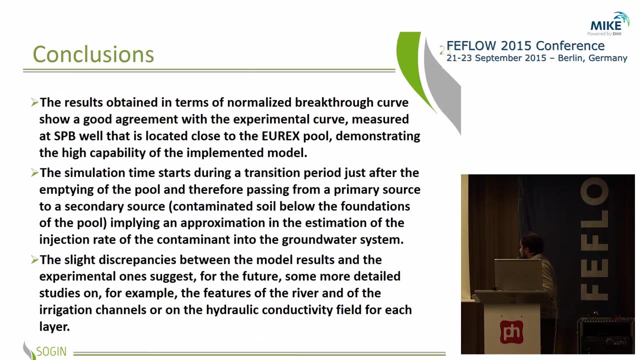 so we have here. we can see the Eurex pool and the point of the release of the source is in the corner of the side of the pool and the some conclusion. the results obtained is a good results, but the difference in the concentration, normalized concentration- between 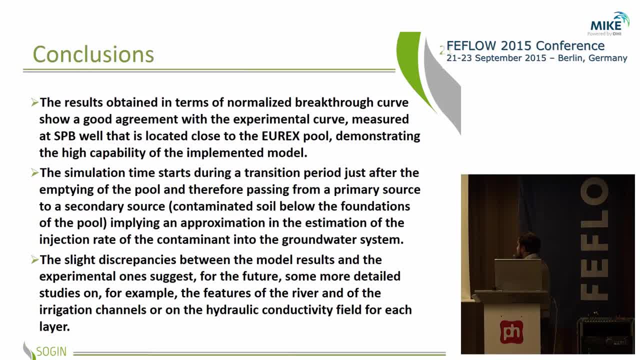 the observed and the calculated curves. it depends, for example, because the simulation time starts during a transition period, just after the empty of the pool and therefore passing from a primary source where the strontium is present and to a second resource, implying approximation in the estimation of the 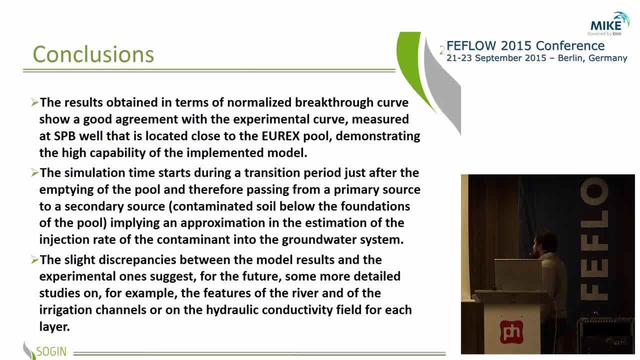 reaction rate of the contaminant to the groundwater system and the slight discrepancies between the model results and experimental ones suggest for the future some more detailed studies, for example for the future of the river and of the irrigation channel, or on an hydraulic conductivity field for each layers. 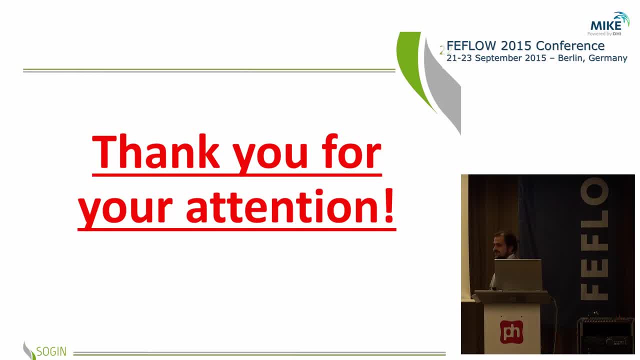 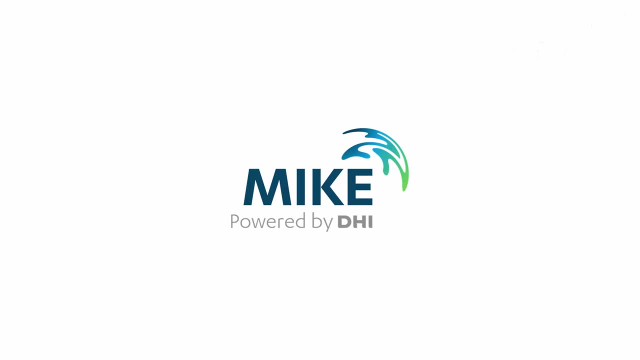 thank you for your attention. you.